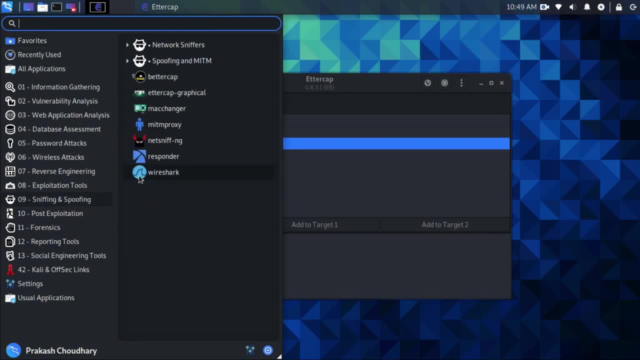 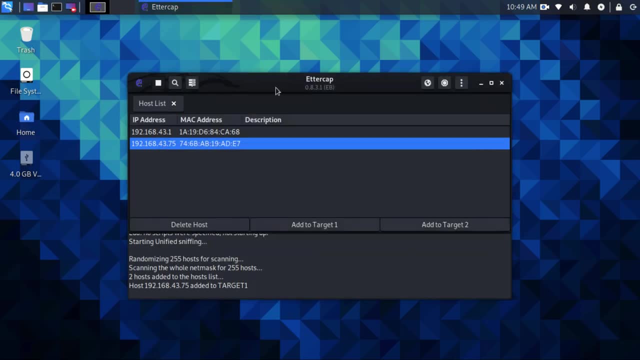 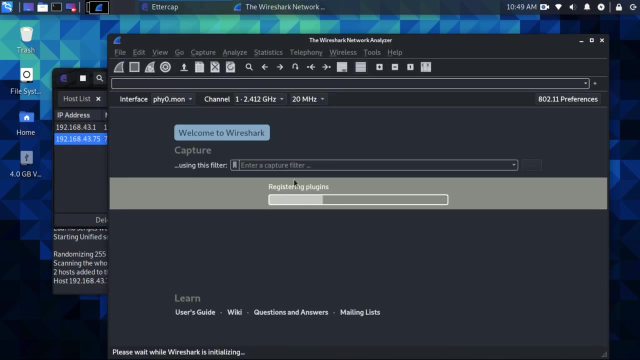 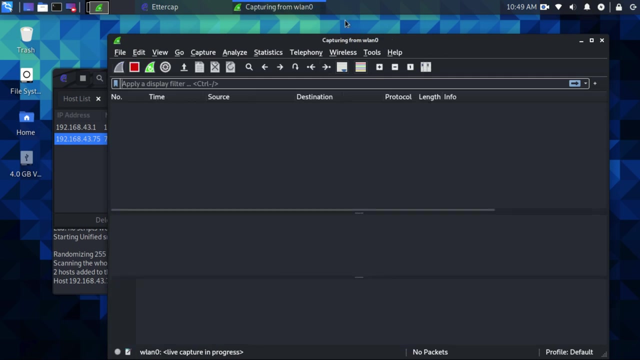 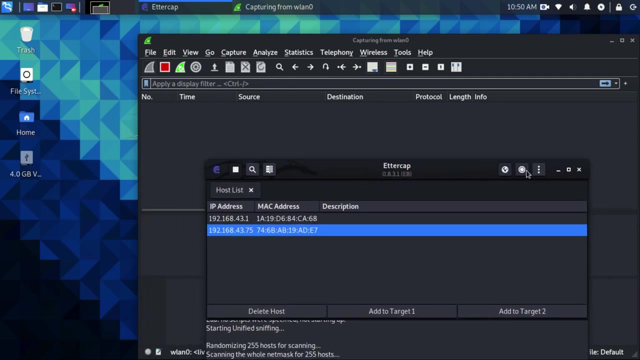 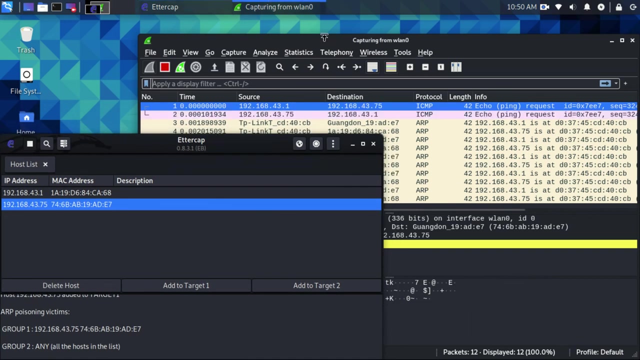 You can open Wireshark to see what's happening on the network. Now click on the ARP Poisoning to see more details. Then click on the ARP Poisoning and you will notice that our interface has now become the gateway. Now click on the ARP Poisoning to see what's happening on the network. 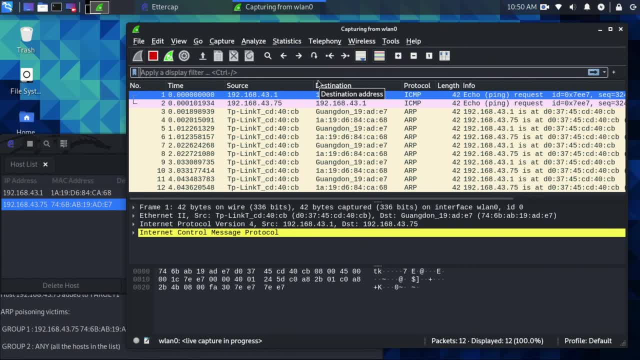 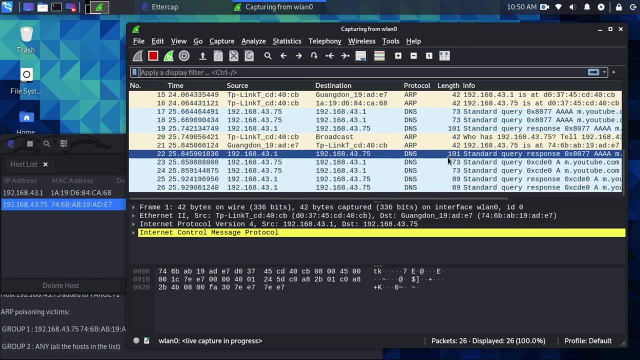 You can now see the network has been changed from the default ARP Poisoning to ARP Poisoning. Now click on the ARP Poisoning to see more details. To check this, I will go to YouTube and the hacked device and you can see the request. 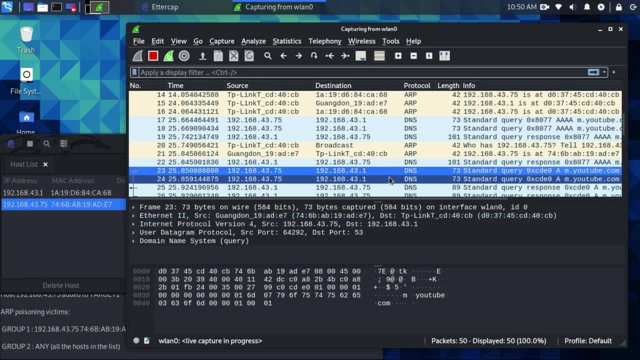 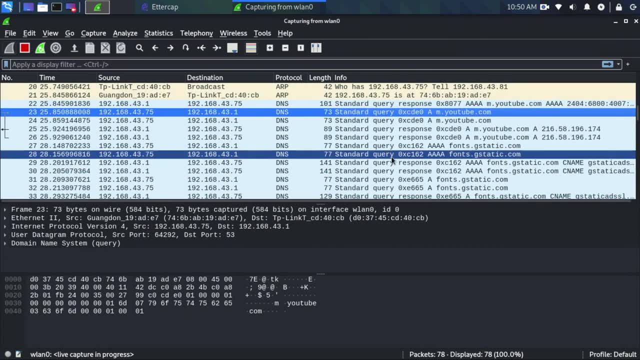 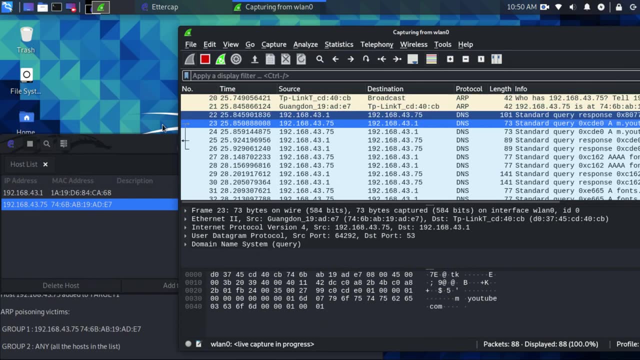 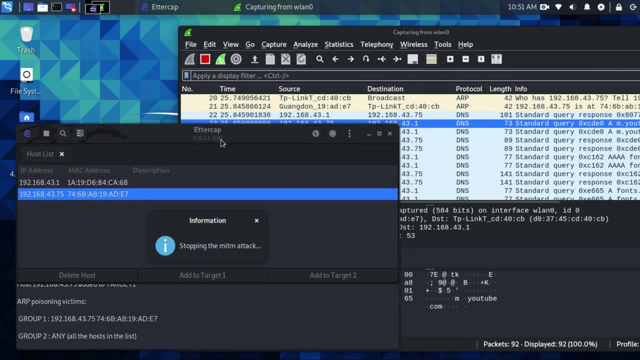 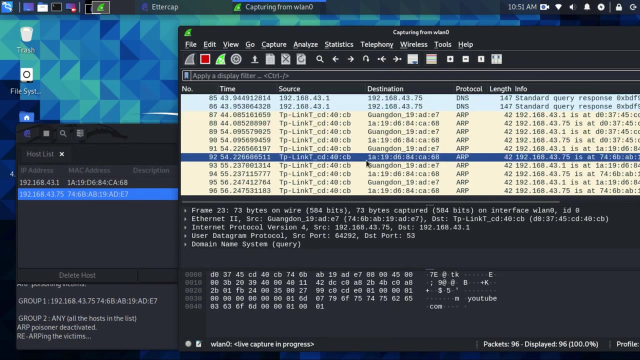 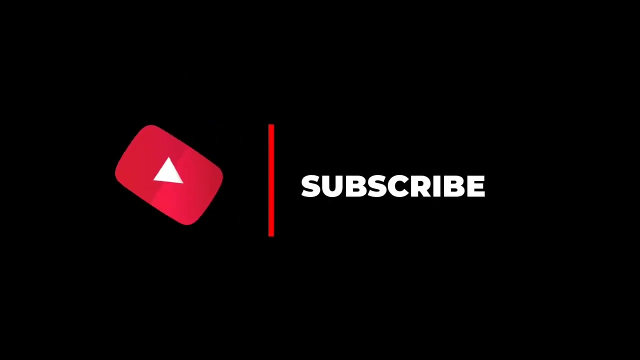 going through my interface To stop this attack. you can click on the stop icon on the window. We will discuss DNS hijacking on next tutorial, So don't forget to subscribe my channel. 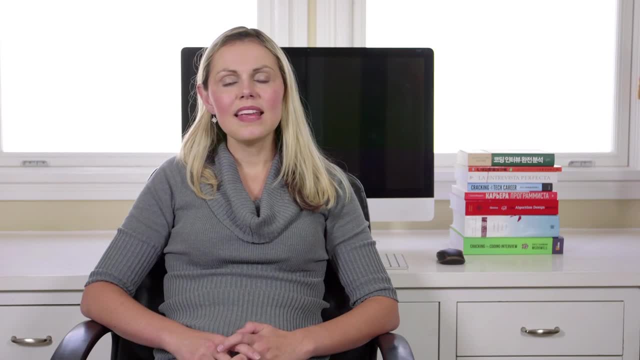 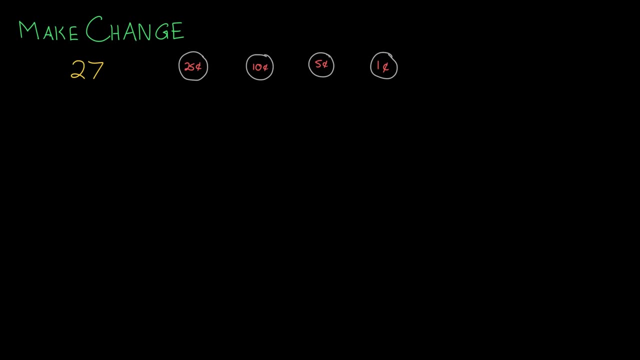 Hi, I'm Gayle Locke-McDowell, author of Cracking the Coding Interview. Today I want to talk about the make change problem. So we want to give someone a certain amount of money and we have a list of all the denominations, And the question is, how many different ways can we do that? 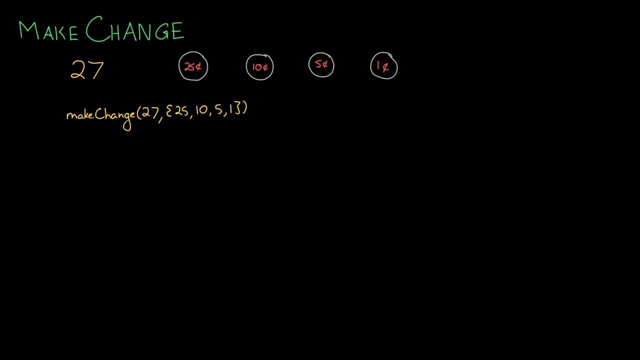 So let's walk through this for a particular possibility. Suppose we want to make 27 cents out of these coins here. Well, the first thing we need to figure out is: well, how many quarters are we gonna give? Are we gonna give one quarter, or are we gonna give zero quarters?